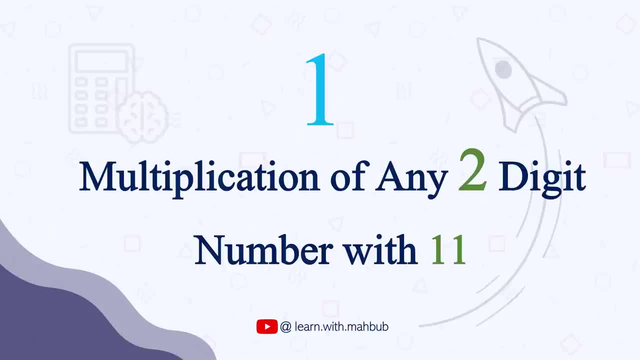 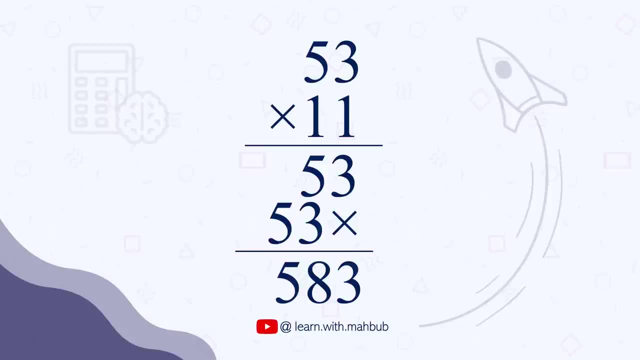 you multiply 53 with 11?? Well, the method we learned in school is easy, but a bit longer. Rather, let me teach you a very cool trick which is even easier. For this, we will keep 5 and 3 of 53 in two sides and then take their sum, 5 plus 3, which is 8 in the middle. 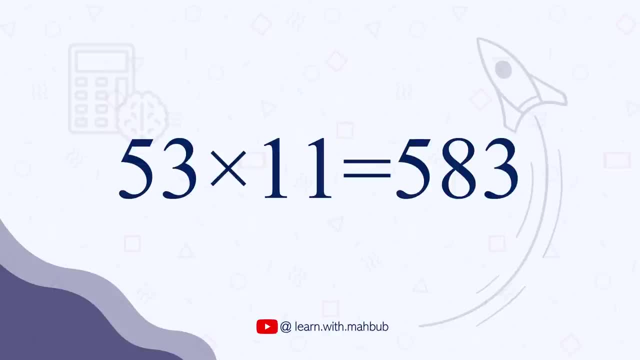 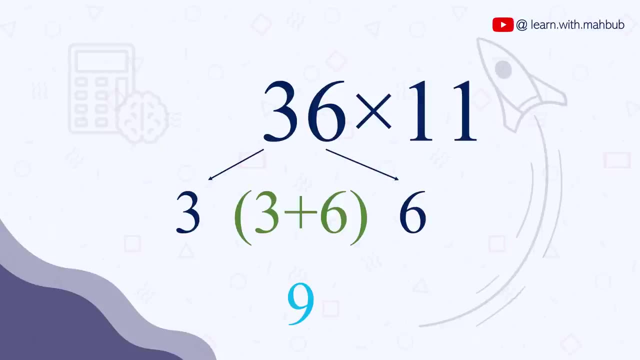 So 53 times 11 is 583.. See, lightening first. Isn't it a cool trick. Let's try some more: 36 times 11.. It is 3.. 3 plus 6 is 9 and 6.. So 396.. As fast as that. 62 times 11 is 682.. 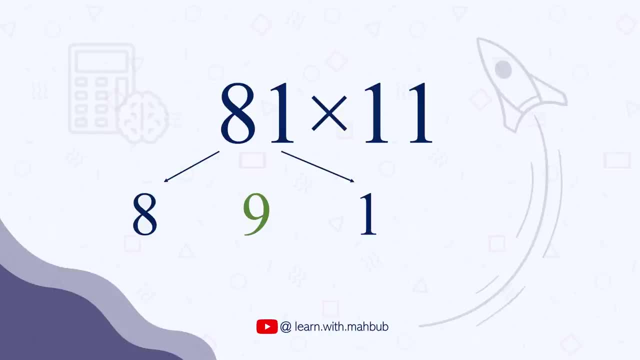 81 times 11 is 891.. You are now faster than a calculator. Now what if the sum is 10 and above, For example 28 times 11.. 2 plus 8 is 10 and 8.. Here, 0 will be in the middle spot and 1 will be the carry. 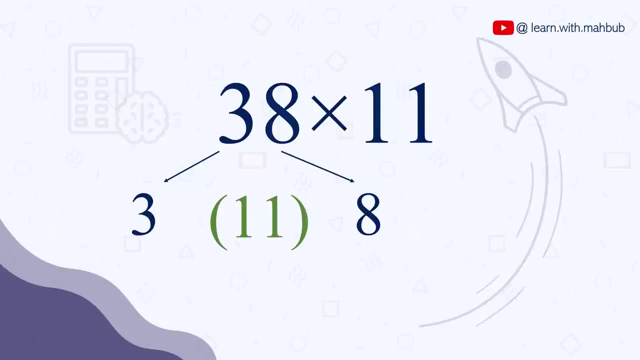 So it will be 308.. Let's try some more: 38 times 11.. 3 plus 8 is 11.. So it will be 418.. Look how fast we are. 79 times 11.. 869.. 84 times 11 is 924.. 99 times 11 is 1089.. That means: 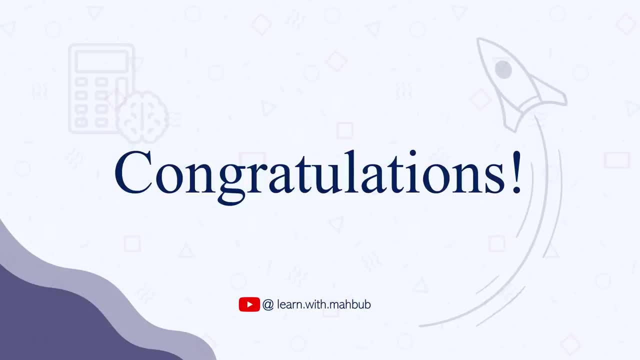 1089.. Congratulations: You can now multiply two-digit numbers with 11 faster than a calculator. Before moving to the next trick, let me show you how to multiply two-digit numbers with 11 faster than a calculator. If you already get any value from this video, please like this video. share with your friends. 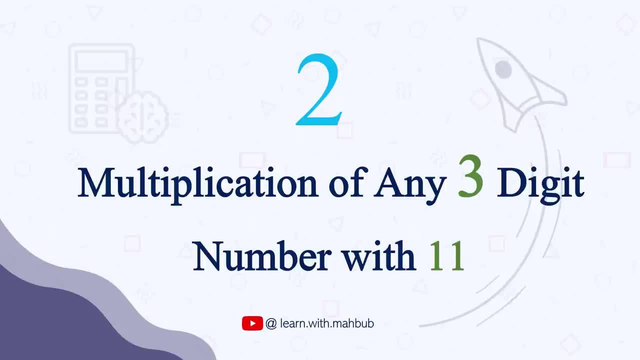 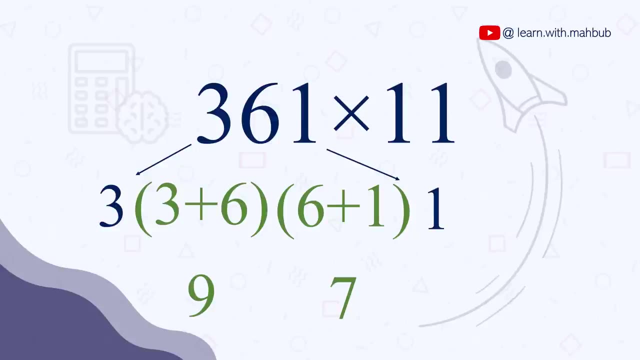 and don't forget to subscribe to this channel. Now trick 2.. Multiplication of three-digit number with 11.. I won't take too much time because the method is almost similar. Let's try some example. 361 times 11. It will be 3.. 6 plus 3 is 9.. 6 plus 1 is 7 and 1.. So 361 times 11 is 3971.. Now 245.. 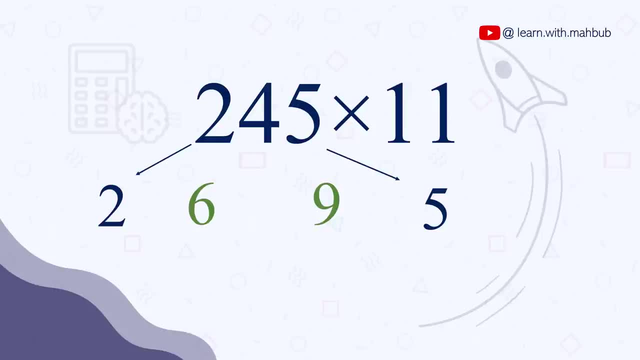 times 11 is 2695.. See, you are lightening. first, Now, if the sum is 10 or above, what do you need to do? You need to use it as carry. For example, 675 times 11 is 6 plus 7 is 13.. 7 plus 5 is 12.. 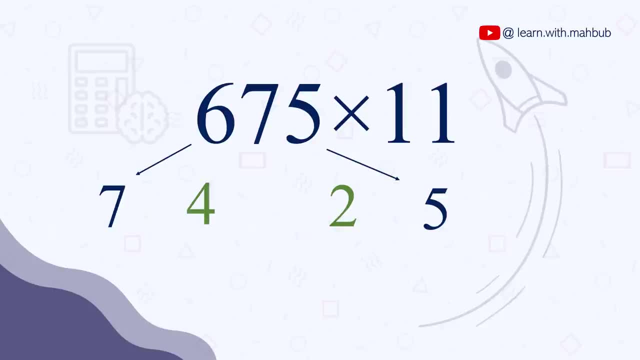 So it will be 7425.. I know, initially you may have some trouble to calculate these carries, but with practice it will be very, very easy. Let's practice two more: 197 times 11.. It will be 2167.. 671 times 11 is 7381.. See, you are now faster than a calculator. 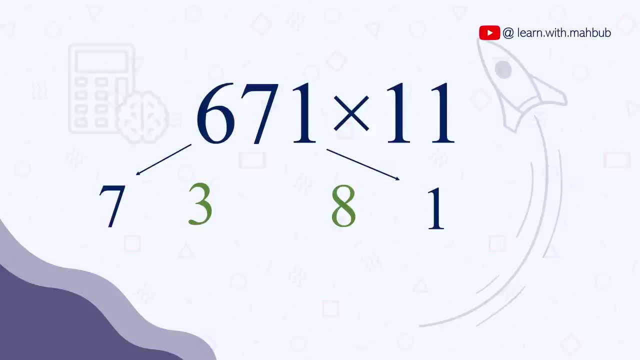 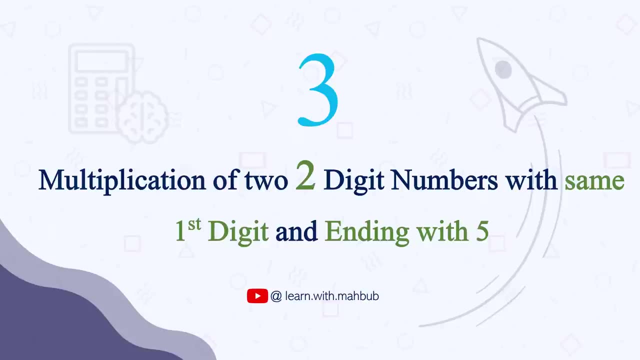 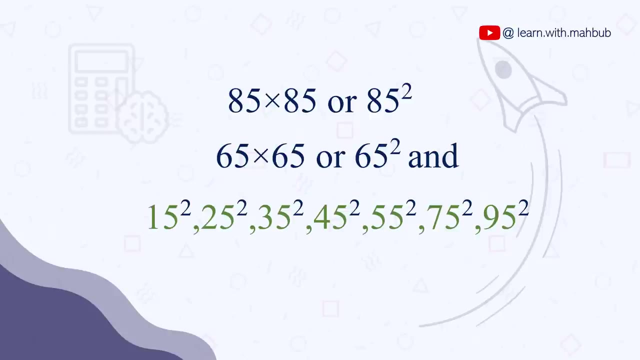 in three-digit number as well, while calculating or multiplying with 11.. Now our third trick is multiplication of any two-digit number, starting with the same digit and ending with 5.. For example, 85 times 85 or 65 times 65. You can do it for 15,, 25,, 35,. 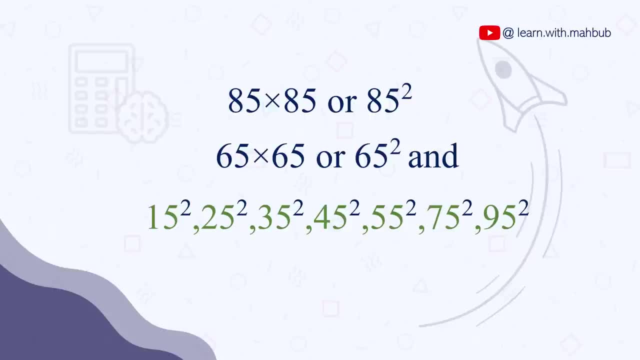 45,, 55,, 75 and 95 as well. So this is not just a multiplication trick, This is also a square trick as well. How to do it? Let's try 85 times 85.. For doing this, you need to multiply the first. 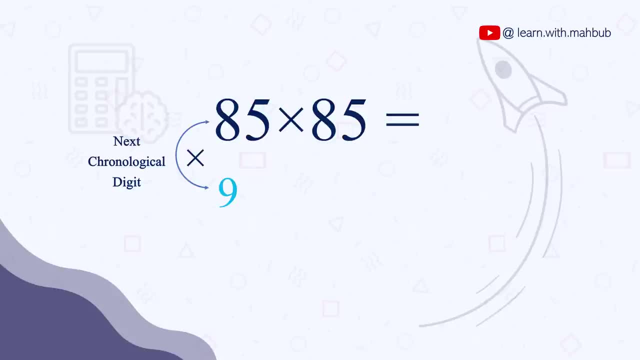 digit, which is 8, in this case, with its next chronological digit, which is 9.. So 9 times 8 is 72.. This was the first part, and then just write 25.. So 85 times 85 is 7225.. As simple as that. 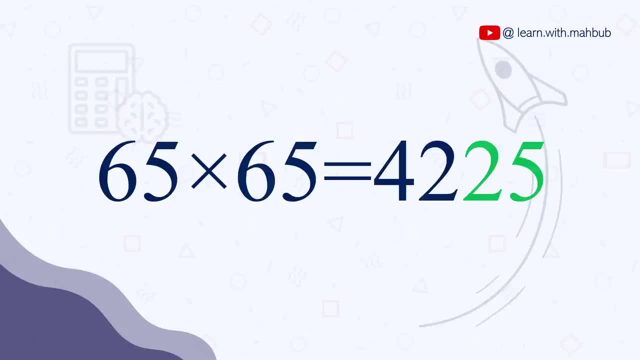 Let's try some more examples. 65 times 65 is 4225.. Here, 42 is the result of 6 times 7.. Let's try some more: 35 times 35, which is 1225.. 45 times 45 is 2025.. 55 times 55 is 3025.. See, you are now faster than a calculator. 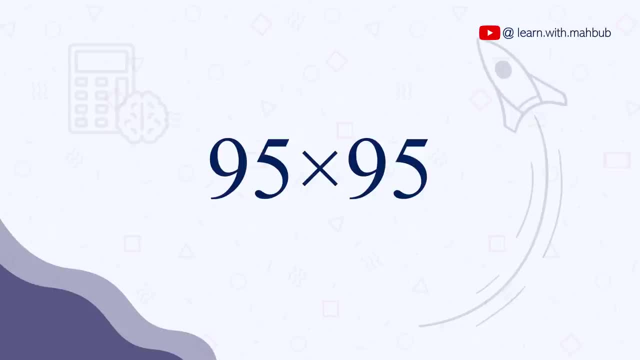 So tell me what is 95 times 95 or 95 square. Very simple: 9 times 10 is 90, and then 25, which will be 9025.. Clear, Can we move to the next trick? Okay, Now moving to the trick 4.. Multiplication of two. 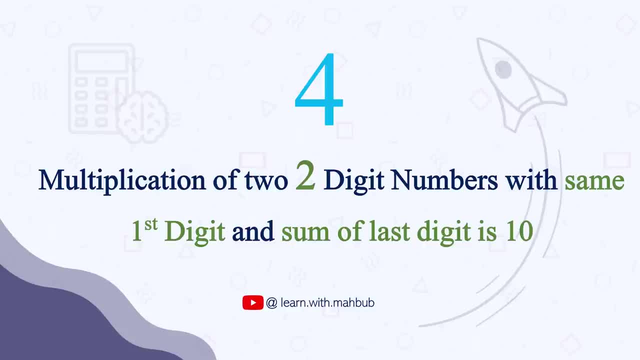 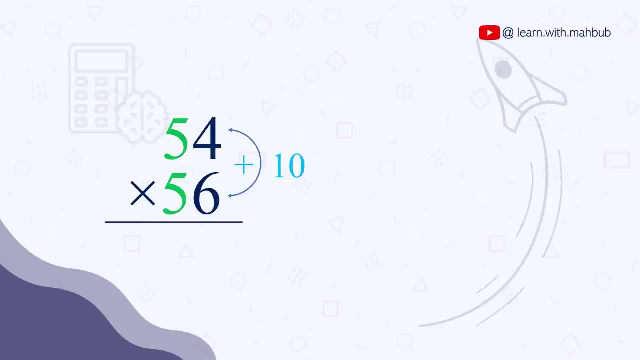 digit number who have same first digit and the sum of large digits are 10.. For example, 54 times 56.. Same first digit, and 6 plus 4 is 10.. 18 times 12.. Same first digit, which is 1. 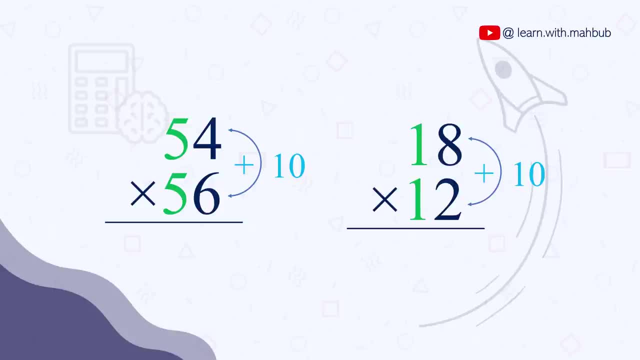 and 8 plus 2 is 10.. How to do these kinds of calculations just in a second First part is the same as previous. For this you need to multiply the first digit with its next chronological digit and then multiply the next two digits. Let's try some example: 73 times 77.. Can you do it in? 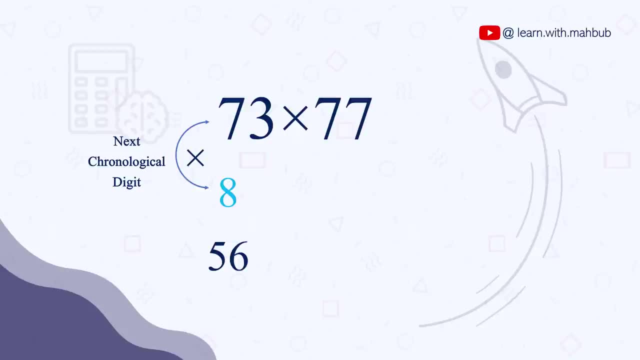 a second. Let's try and comment down below. Let's see how to do it. The next digit of 7 is 8.. So 7 times 8 is 56, which is the first part. Then multiply the last digits 3 times 7 is 21.. So 73 times 77 is. 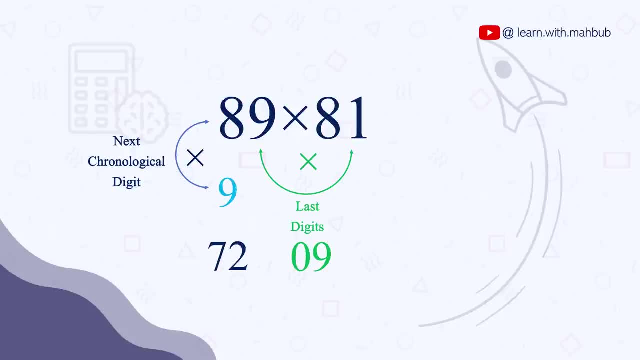 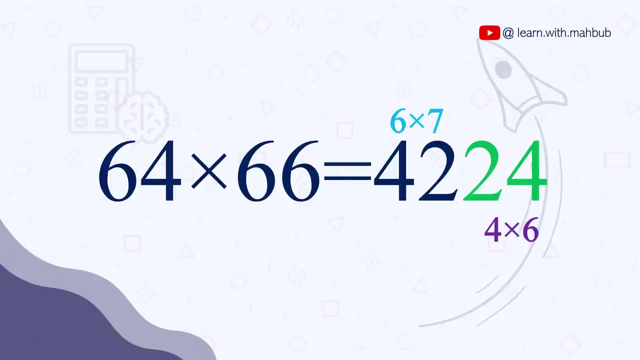 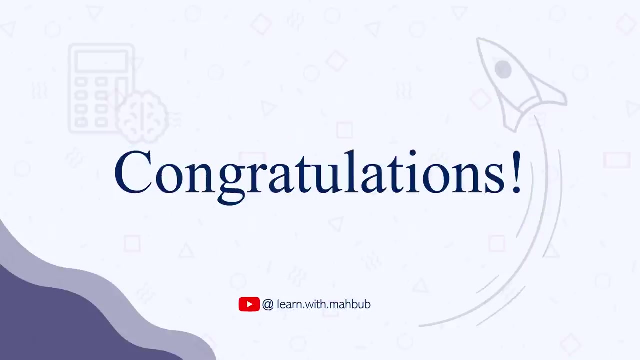 21.. As simple as that. Let's try some more example: 89 times 11.. It is 70 to 09.. 64 times 66.. 40 to 24.. 18 times 12 to 16.. 37 times 33.. 12 to 21.. See, you are already doing calculations like. 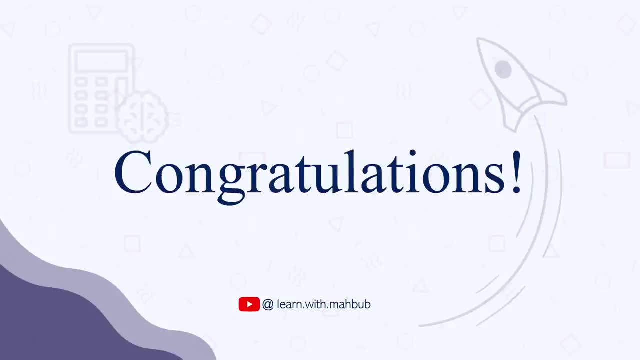 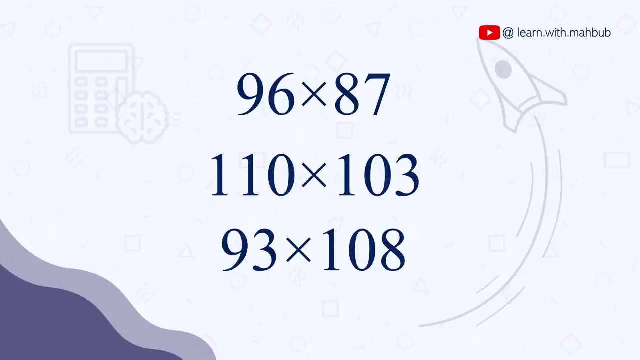 a human calculator faster than a machine calculator. Now the final trick for today is to multiply any number near by 100.. It can be 96 times 87. It can be 10 times 103.. Or it can be 93 times 108.. Let me tell you the answers first. 96 times 87 is 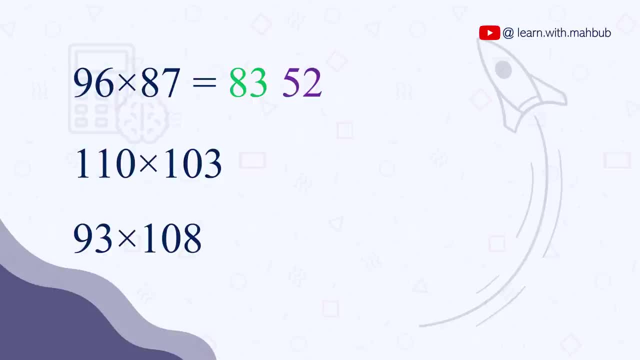 8352.. That means 8352.. 110 times 103 is 11330.. That means 11330.. 93 times 108 is 144, which means 10044.. What do you think? Are you interested to learn this? 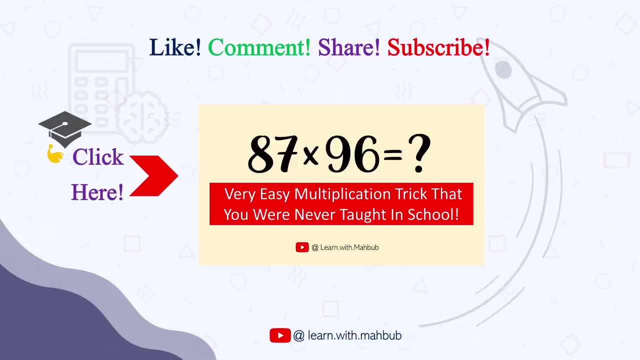 technique. Please comment down below. Thanks for watching. I have a dedicated video on this trick, which is the most viewed video of this channel so far. You can just click here in the middle or in the card and watch this video and, if you have, 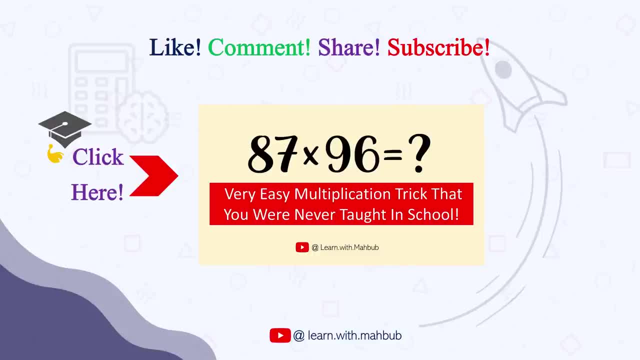 already watched this video. thank you so much for your love. Please subscribe to this channel for the next video of this series and comment me which trick you liked most.